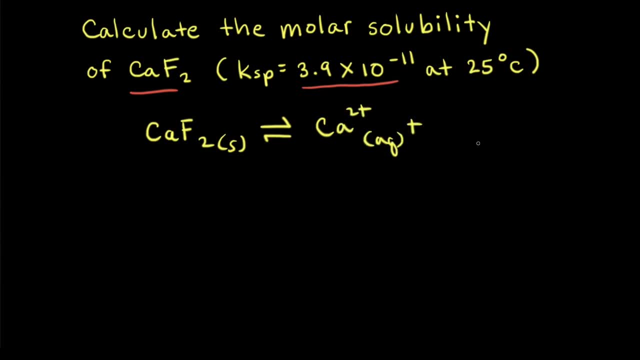 calcium 2 plus ions and fluoride anions and to balance that out, we need to make sure and include a 2 in front of the fluoride anions. The next step is to set up an ICE table, where I stands for initial concentration, C stands for the change in concentration and E stands for equilibrium. 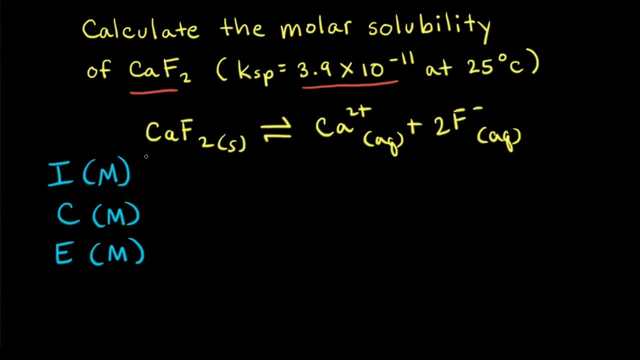 concentration Before any of the solid calcium. fluoride dissolves. the initial concentrations of calcium 2 plus ions and fluoride anions in solution is zero. So we can go ahead and put a zero in here for the initial concentration of the ions in solution. Some of the calcium 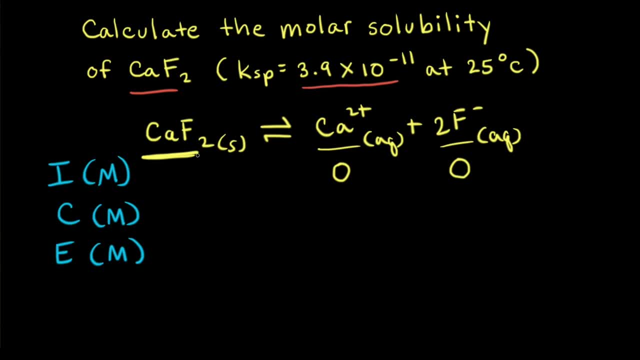 fluoride anions and fluoride anions dissolve in solution. Some of the calcium fluoride anions will dissolve, and we don't know how much, so I like to represent that by writing minus x on the ICE table, where x is the concentration of calcium fluoride that dissolves. Looking at the mole, 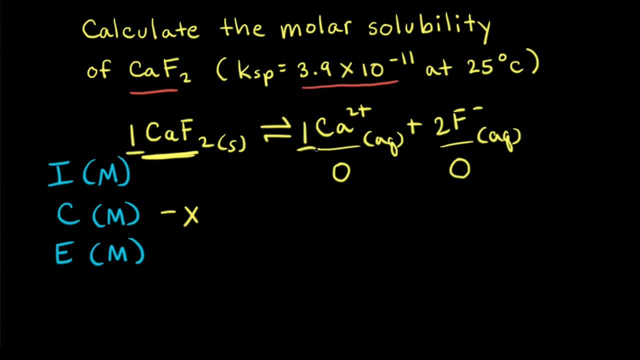 ratios. it's a one to one mole ratio between calcium fluoride and calcium 2 plus ions. So if we're losing x for the concentration of calcium fluoride, we must be gaining x for the concentration of calcium 2 plus ions. And since it's a one to two mole ratio for calcium 2 plus ions to fluoride and 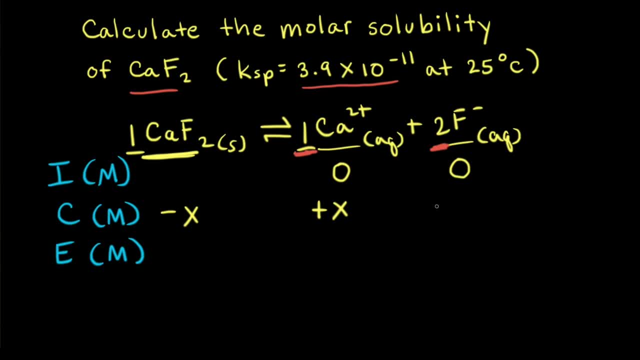 ions. if we're gaining plus x for calcium 2 plus, we must gain plus 2x for fluoride anions. So the equilibrium concentration of calcium 2 plus ions is zero plus x or just x, and the equilibrium concentration of fluoride anions would be 0 plus 2x or just 2x. The next step is to write the Ksp. 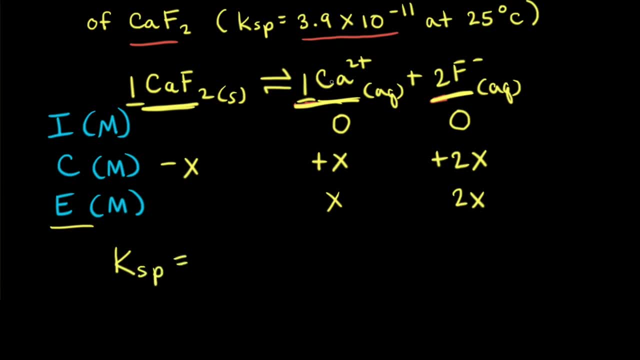 expression from the balanced equation. So Ksp is equal to the concentration of calcium 2 plus ions and since there's a coefficient of one in the balanced equation, it's the concentration of calcium 2 plus ions raised to the first power times, the concentration of fluoride anions. and 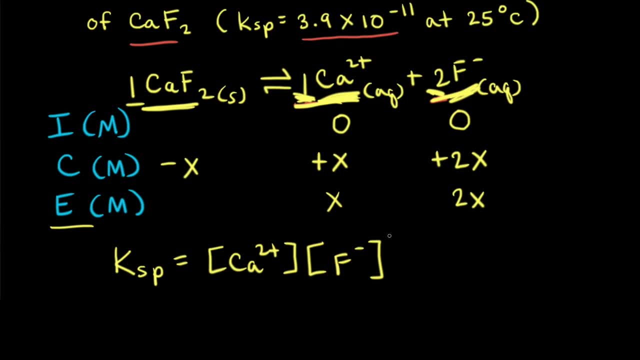 since there's a coefficient of two in the balanced equation, it's the concentration of fluoride anions raised to the second power. Pure solids are not included in equilibrium constant expressions, so we're going to leave calcium fluoride out of the Ksp expression. The concentration of ions in our 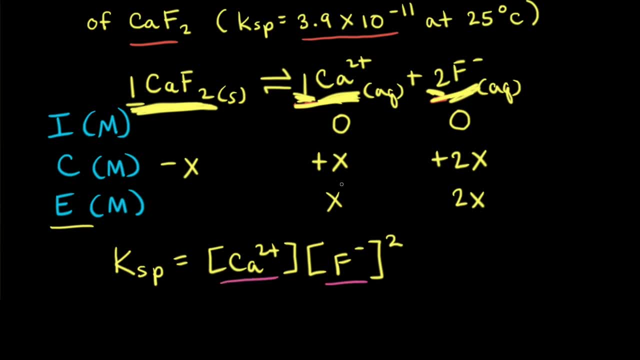 Ksp expression are equilibrium concentrations. Therefore we can plug in x for the equilibrium concentration of calcium 2 plus and 2x for the equilibrium concentration of fluoride anions. We can also plug in the Ksp value for calcium fluoride, So that would give us 3.9 times 10 to the negative. 11th is equal to x times 2x squared. 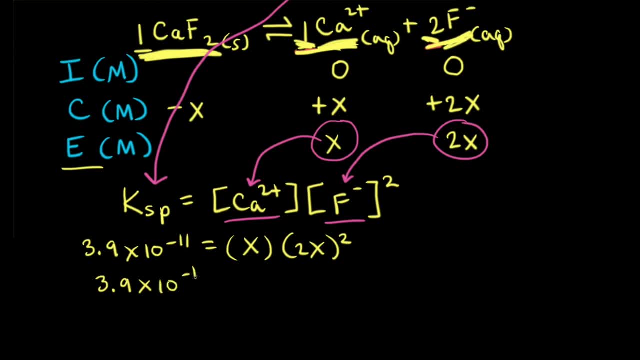 Next we need to solve for x. so 3.9 times 10 to the negative 11th is equal to x times 2x squared. Well, 2x squared is equal to 4x squared times x is equal to 4x cubed. 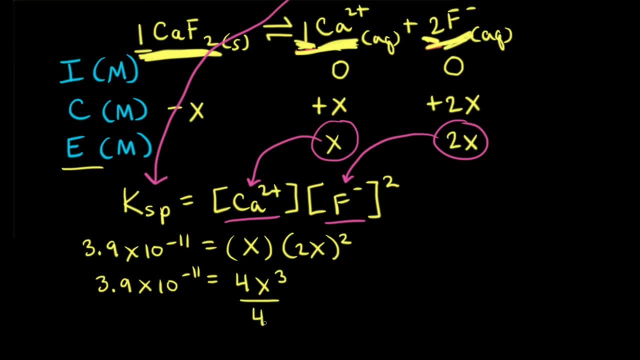 So to solve for x, we need to divide both sides by 4 and then take the cube root of both sides. So we take the cube root of the left side and the cube root of x. cubed, That gives us x is equal to 2 x squared and 2 x squared squared. See, because we've got the same value. we're going to 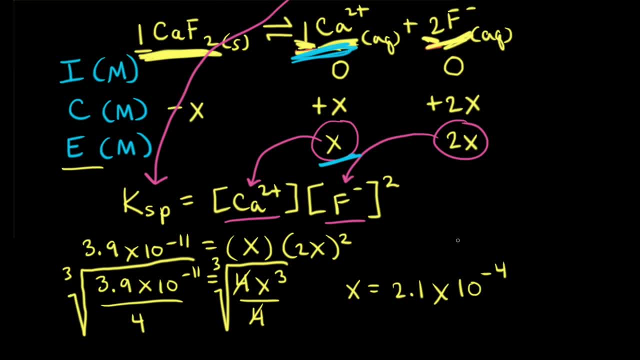 square them to the left to create 1.. tight square Based on both dimensions. we can call this equation a: 1 to the minus per ogles cost. So x times 2.1, times 10 to the negative, 0.4 is the equilibrium. 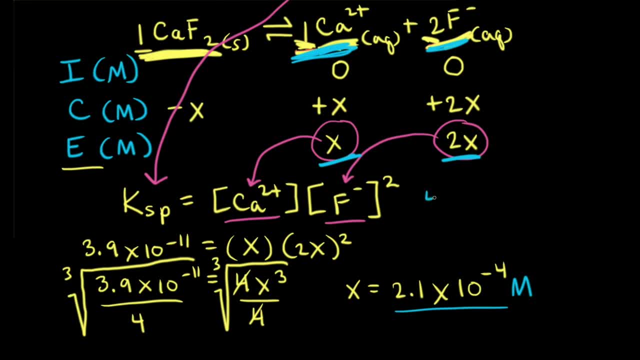 concentration of calcium 2 plus ions. The equilibrium concentration of calcium 1 plus ions is 2.1 times of fourth molar for the equilibrium concentration of fluoride anions. Our goal was to calculate the molar solubility of calcium fluoride. 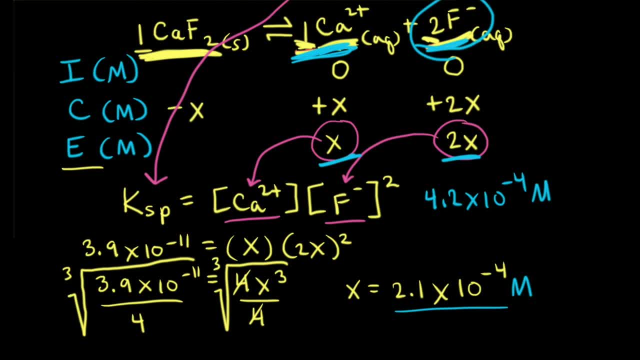 And molar solubility refers to the concentration of our salt that dissolved to form a saturated solution at equilibrium. So if X refers to the concentration of calcium two plus ions at equilibrium, looking at our mole ratios, that's also the concentration of calcium fluoride. 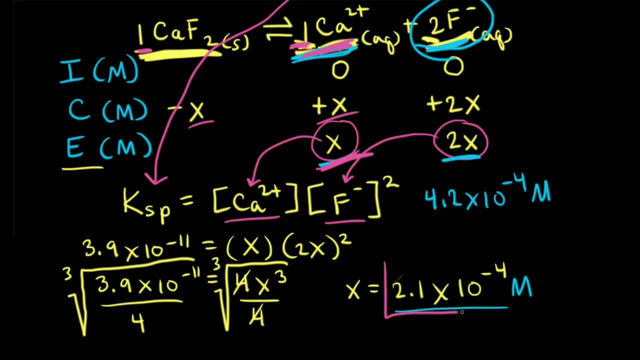 that dissolved, Therefore 2.1 times 10 to the negative. fourth molar is also the molar solubility of calcium fluoride. Technically, at a constant temperature of 25 degrees, the concentration of a solid doesn't change, And so you'll see most textbooks not put in minus X. 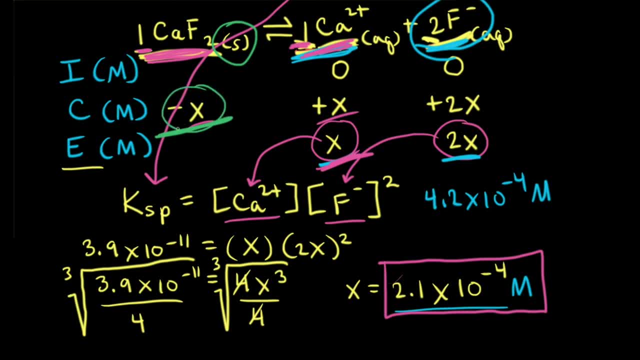 on the ice table. I like to just put it in, though, to remind me that X, in this case, does refer to the molar solubility.